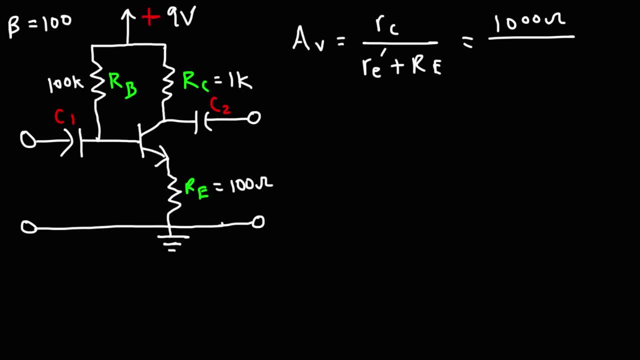 And before we can do that we need to calculate IE. By the way, the AC emitter resistance is equal to 25 millivolts divided by IE. Now, before we can calculate the emitter current, we need to calculate VE, the emitter voltage with respect to ground, and before we can do that we need to calculate VB and before that, IB. 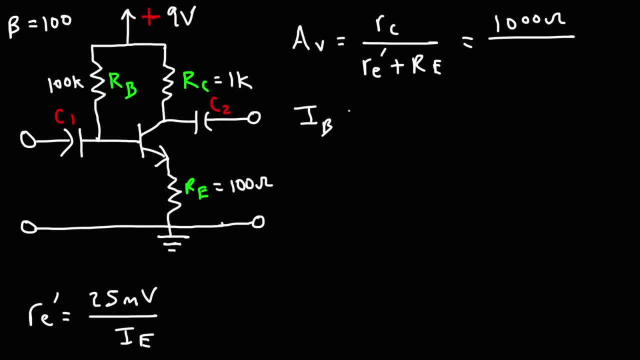 So let's calculate the base current first For this particular circuit. this is the formula that you need to calculate the base current. It's VCC minus VBE, divided by RB Plus beta plus one times RE. Now for those of you who might be interested in how I got that formula, there's another. 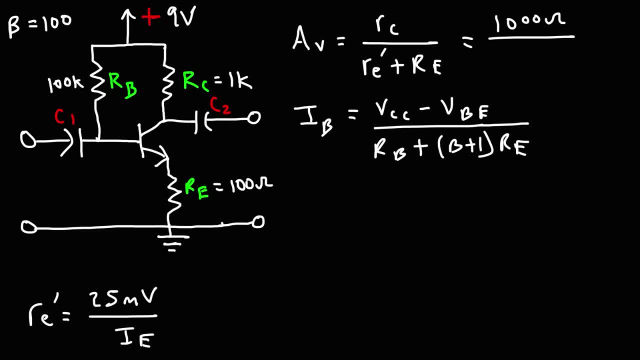 video that I created on YouTube entitled emitter feedback bias circuit, which explains how to derive that formula. For those of you who are interested, check out the links in the description section below of this video, because I'll post that video in that area so you can quickly take a look at that. 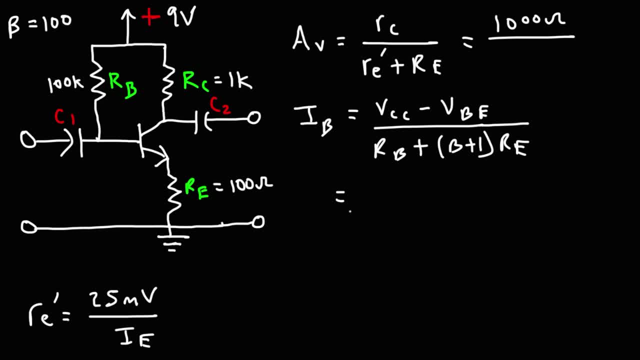 If you're wondering where to get this formula Now: VCC: the collector supply voltage, that's nine volts. VBE: the voltage between the base and the emitter of the transistor, that's typically 0.7 volts. The base resistor: RB, that's a hundred kilo ohms. 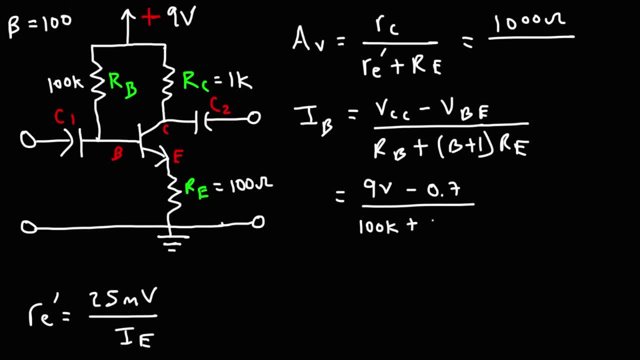 Beta for this transistor is a hundred. so beta plus one, that's 101.. Now RE is a hundred ohms, but because RB is in kilo ohms we want the units to match, So we're going to convert that to kilo ohms. 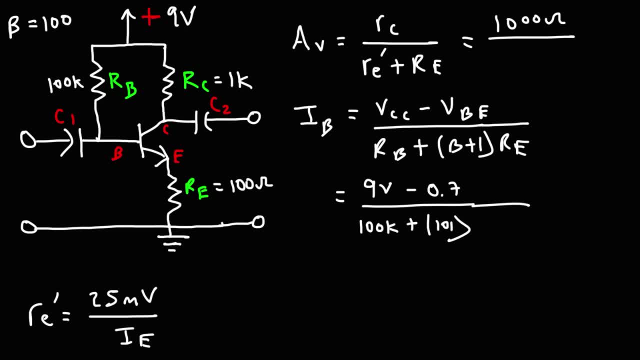 To convert ohms into kilo ohms, divide by a thousand. A hundred divided by a thousand is 0.1.. So RE is 0.1 kilo ohms. So we have nine minus 0.7. that gives us a voltage of 8.3 volts, and then 100 plus 101 times 0.1.. 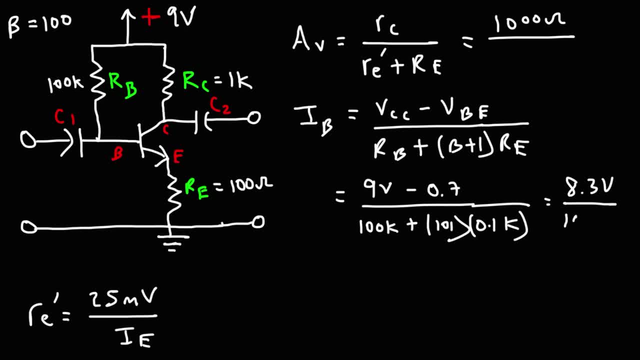 Gives us a total AC resistance- AC emitter resistance- of 110.1 kilo ohms. So 8.3 divided by 110.1, that's going to be 0.0754 milliamps. When you divide volts by kilo ohms you're going to get the current in milliamps. 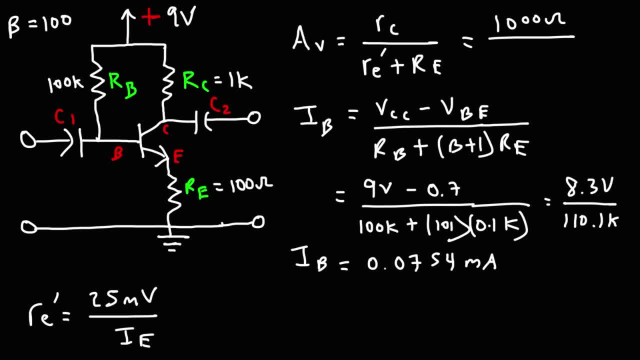 Now there's many ways in which you can calculate IE given IB. As I mentioned before, you can calculate VB, VE and then IE, But this is an easier way of calculating IE from IB Instead of going through all those steps. IE is the sum of IC and IB. 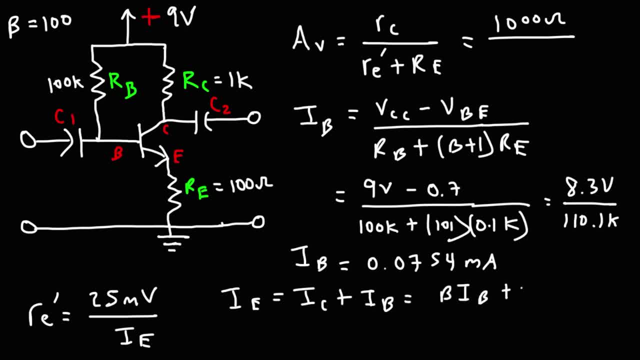 And IC is beta times IB. So if you factor out IB, IE is basically IB times beta plus 1.. So that's going to be 0.0754 milliamps times 100 plus 1, or 101.. So that's IE which I'm going to write here. That's 7.615 milliamps. 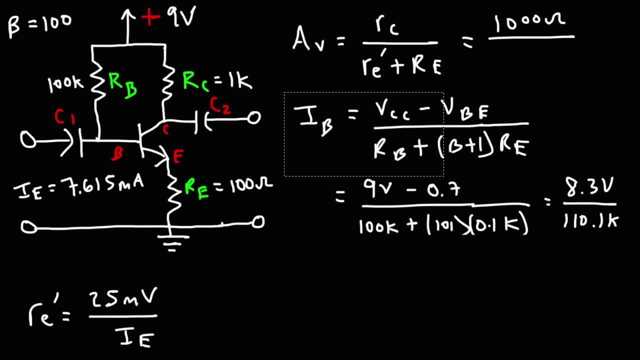 So now that we have the value of IE, we can now calculate the AC emitter resistance. So it's 25 millivolts divided by 7.615 milliamps. So 25 divided by 7.615, this will give us a resistance of 3.28, but we'll round it to 3.28.. 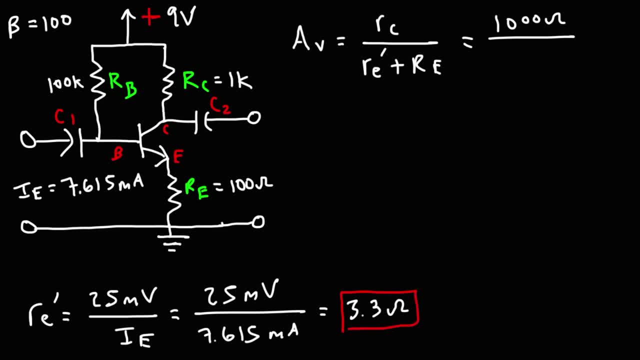 3.3 ohms. So now we can calculate the voltage gain. The AC emitter resistance is 3.3, and RE is 100.. So the voltage gain, that is the ratio between the output voltage and the input voltage that's applied here. 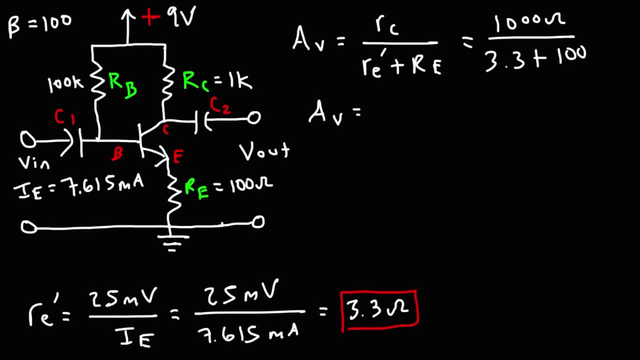 that's going to be 1,000 divided by 1,000, divided by 103.3.. And so you can round that to 9.7.. So that's going to be the voltage gain of this particular circuit. Now there's one more thing I do want to mention regarding this particular circuit. 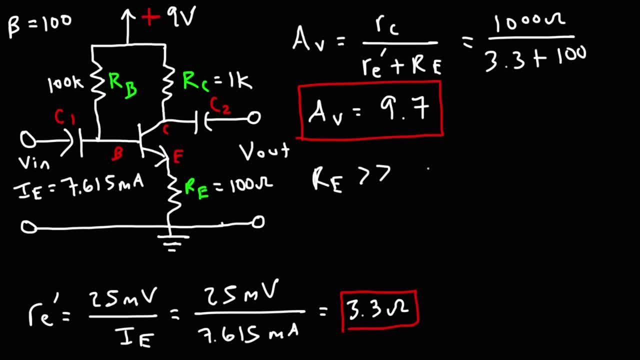 and that is that RE is significantly larger than the AC emitter resistance. When that happens, you can approximate the voltage gain And, assuming that RL is infinity or much higher than RC, the voltage gain is approximately equal to RC over RE, And that's a quick and simple way to approximate the voltage gain. 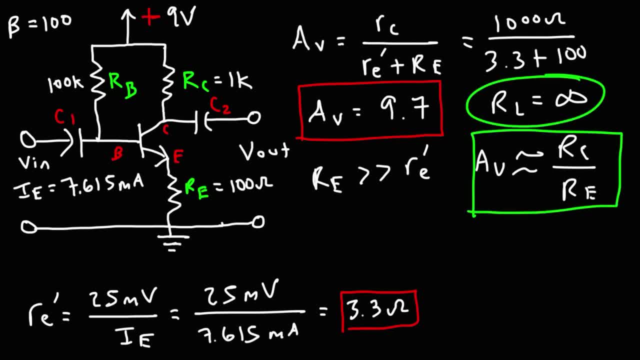 if the load resistance is very, very high relative to RC and if RE is significantly higher than the AC emitter resistance. Notice what the approximation is. Notice what the approximation is. So what we are going to see is what the approximation will be. 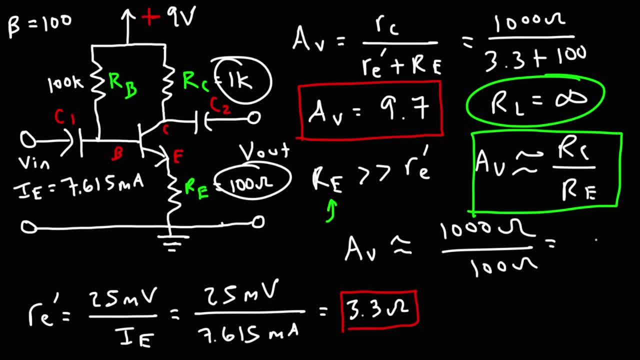 So if we take our one kOhm resistor, which is 1,000 Ohms, and divide it by 100 Ohms, we'll get a voltage gain of around 10, So it's a quick and simple way to estimate what the voltage gain will be. 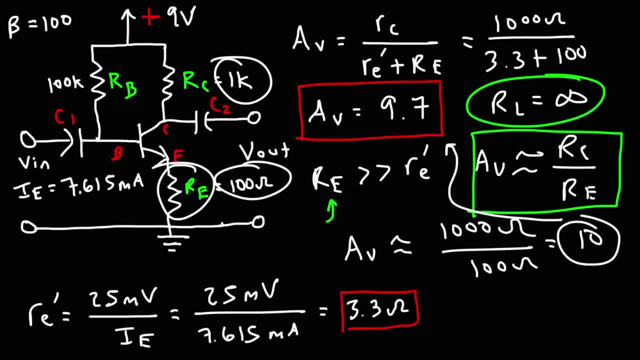 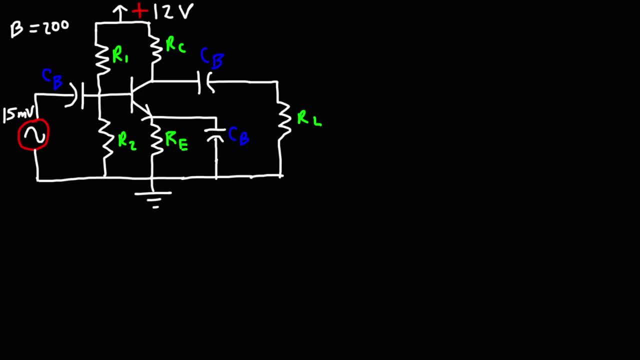 if you have an emitter resistor that is significantly higher than the AC emitter resistance. Now in this example problem we have the voltage divider bias circuit. Now in this example problem we have the voltage divider bias circuit. beta for the transistor is 200 and we're going to say that RC is 510 ohms for this problem. 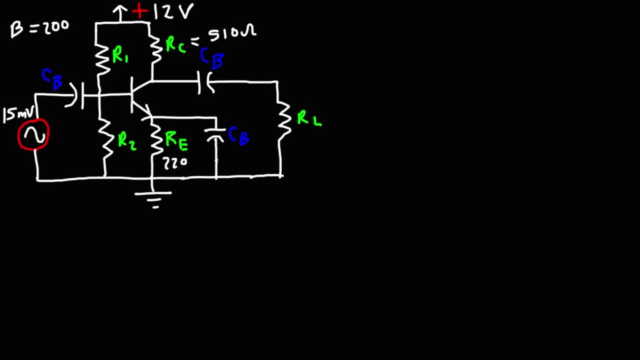 RE is going to be a 220 ohm resistor, R2- we're going to set that to 47 kilo ohms and R1 is going to be 220 kilo ohms. now we do have a load resistor for this problem and we're going to make 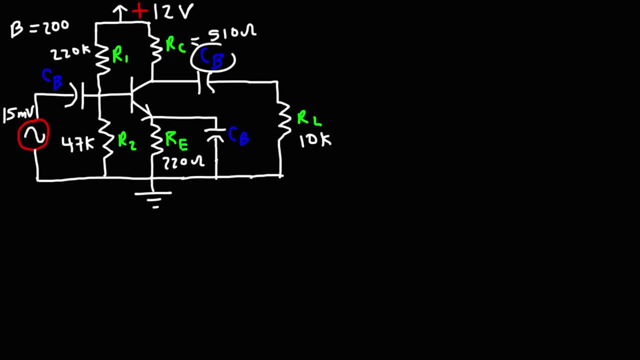 it 10 kilo ohms. CB is the bypass capacitor and for each one we're going to make it 1000 micro farads so that it doesn't introduce any significant capacitive reactants to the circuit. go ahead and calculate the voltage gain of this amplifier and, given the input voltage of the signal, when the 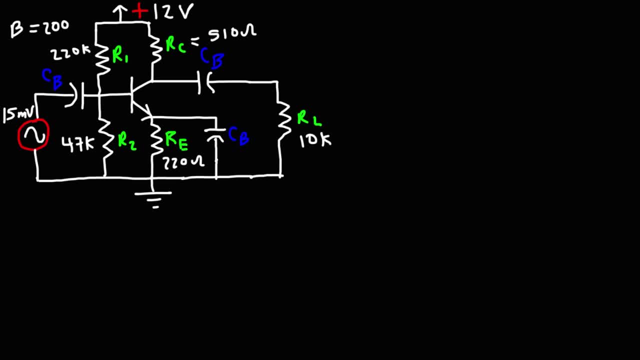 source is connected to the circuit. calculate the output voltage across the load resistor. feel free to pause the video and try this now. the first thing that we need to do is we need to calculate the base current and the formula that we need to calculate the base current given a voltage. 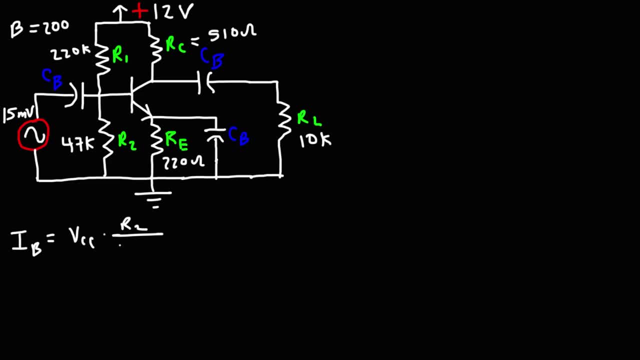 divider by a circuit like what we have here. it's VCC times R2 over R1 plus R2, minus VBE, divided by R2 times R1 over R2, R1 plus R2, and then plus beta plus 1 times RE. 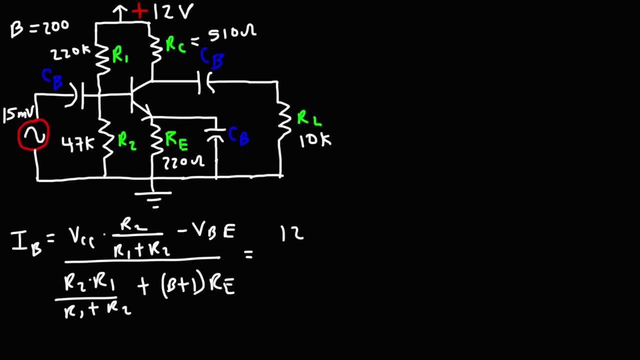 So let's plug in everything that we have. The collector supply voltage is 12, R2 is 47 kilo ohms and the sum of R1 and R2, that's going to be 267 kilo ohms. VBE, as always, will be 0.7, and then R2 times R1.. 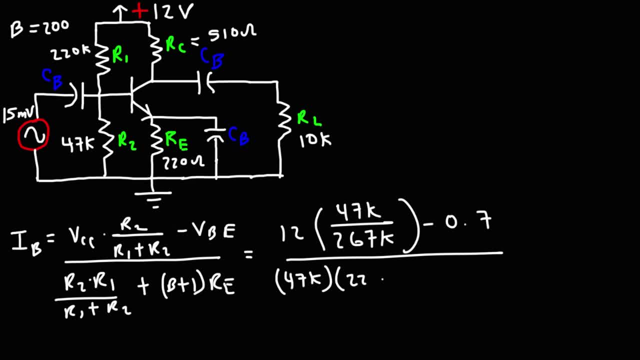 So 47 kilo ohms times 220 kilo ohms divided by the sum of those two, which is 267.. And then beta plus 1.. Beta in this example is 200.. So we have 201 times RE and we want RE to be in kilo ohms. 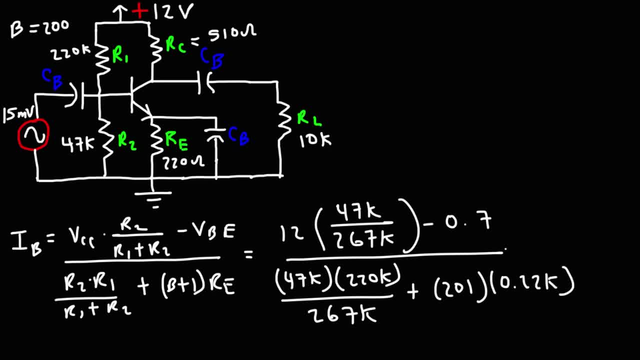 So dividing that by 1,000, that's going to be 0.22 kilo ohms. So 12 times 47 divided by 267.. Minus 0.7, that gives us a voltage of 1.412 volts. 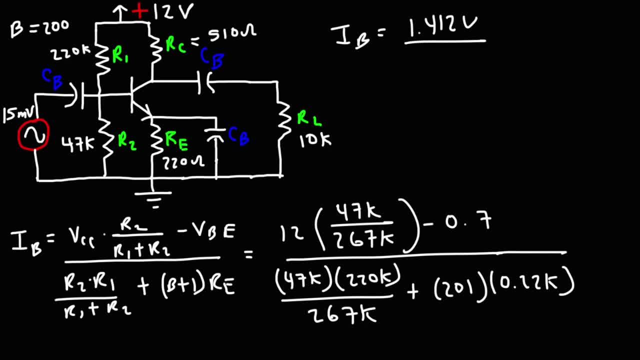 And then 47 kilo ohms times 220 kilo ohms, divided by 267 kilo ohms, that's 38.73 kilo ohms, And then plus 201 times 0.22, we're going to get 82.95 kilo ohms. 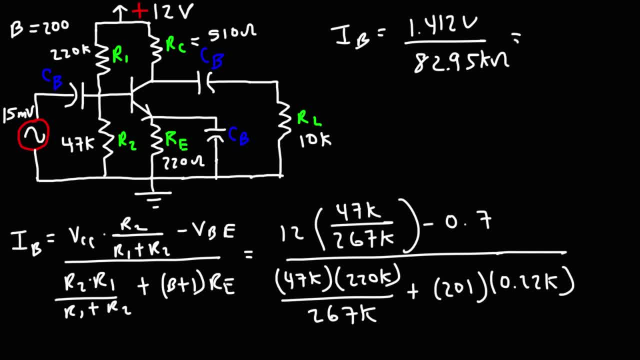 Volt Volt's divided by kilo ohms, so it'll give us the current in milliamps, So 1.412 divided by 82.95.. This gives us a base current of 0.017 milliamps. So that's how we can calculate the base current in this example. 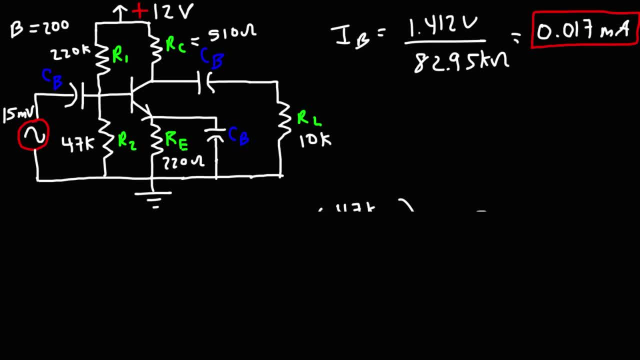 Now that we have the base current, we can now calculate the emitter current And, as we know, the emitter current is equal to beta plus 1.. So beta plus 1, that's 201.. IB is 0.017 milliamps. 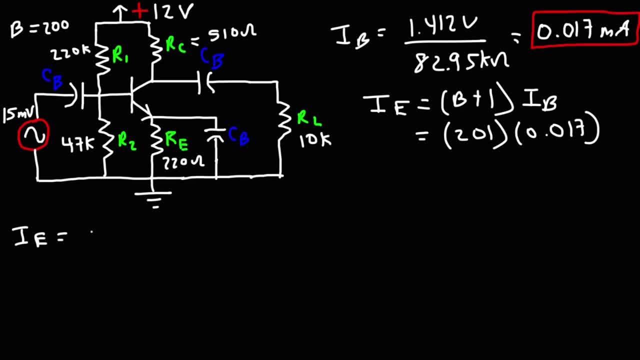 So the emitter current is 3.417 milliamps. So now that we know the emitter current, we can calculate the AC resistance. The AC resistance is going to be 25 millivolts divided by the emitter current. When you divide volts by milliamps you're going to get the resistance in ohms. 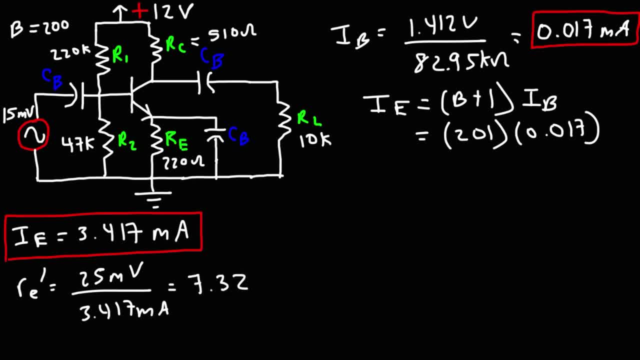 So the AC emitter resistance is 7.32.. Now the voltage gain is going to be RC over the AC emitter resistance plus the emitter resistor. Now let's calculate RC. RC is going to be the parallel combination of that RC and RL. 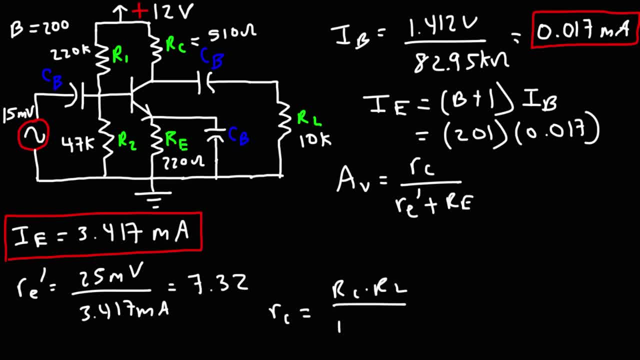 So it's RC times, RL divided by the sum of those two, Because this time we do have a load resistor and we need to take that into account. So RC in this example is 510 ohms. RL is in kiloohms, but we need the units to match. So to convert kiloohms, we need to take the units to match. So to convert kiloohms, we need to take the units to match. So to convert kiloohms to ohms, multiply by 1,000.. 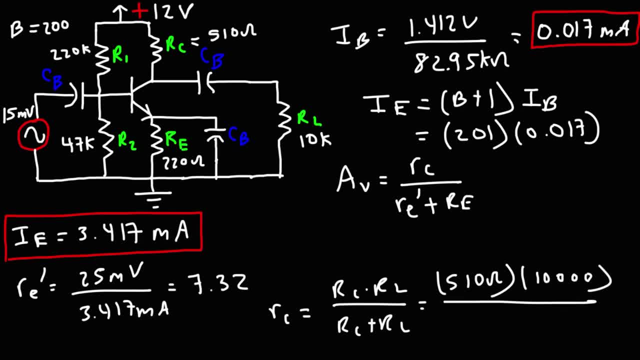 So RL is 10,000 ohms And then the sum of RC and RL, that's 10,510 ohms. So thus RC is 485.3 ohms. Now notice that we have a bypass capacitor across RE And since the bypass capacitor is 4.3 ohms, 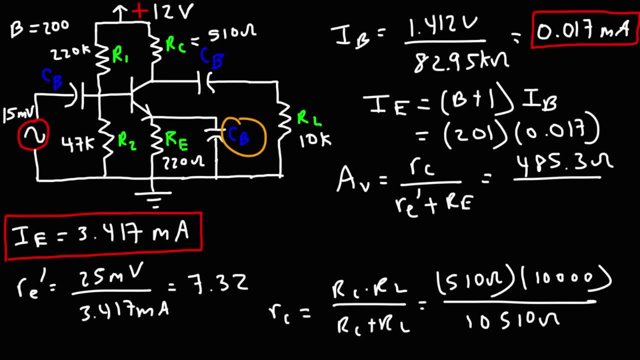 and since the bypass capacitor is 1,000 microfarads, it basically shorts RE when an AC current passes through it. So RE provides resistance to the DC component that goes through it, but the AC component will effectively bypass RE. So thus we can ignore the effect of RE. 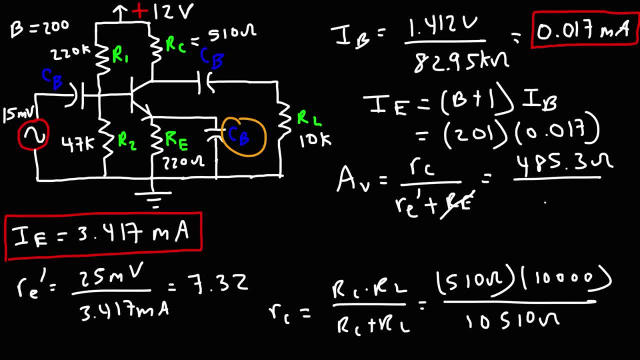 It won't have any effect on the voltage gain of this circuit. So all we need to do is put the AC emitter resistance of 7.32 here, So it's 485.3 divided by 7.32.. Thus the voltage gain for this circuit is 66.3.. 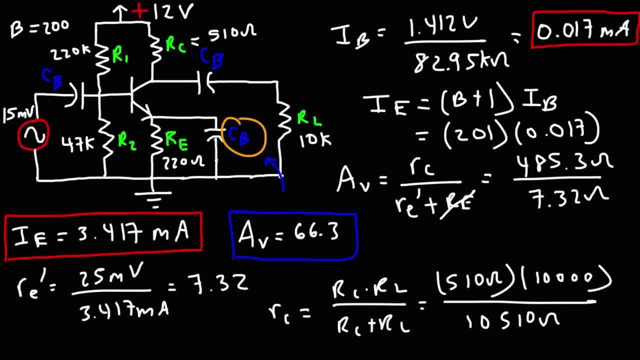 So notice the effect of the bypass capacitor. It increases the voltage gain of the circuit by decreasing the overall AC emitter resistance. Now let's look at the AC emitter resistance. Now let's calculate the output voltage of this circuit. since we know the input voltage, 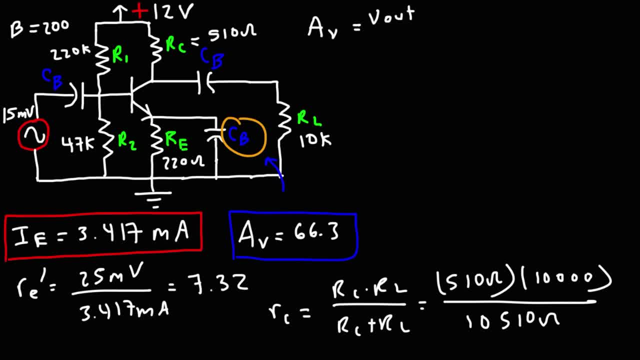 The voltage gain is the ratio of the output voltage to the input voltage. So to calculate the output voltage, multiply the input voltage by the voltage gain. So for this circuit we have an input voltage of 15 millivolts And we're going to multiply it by 66.3.. 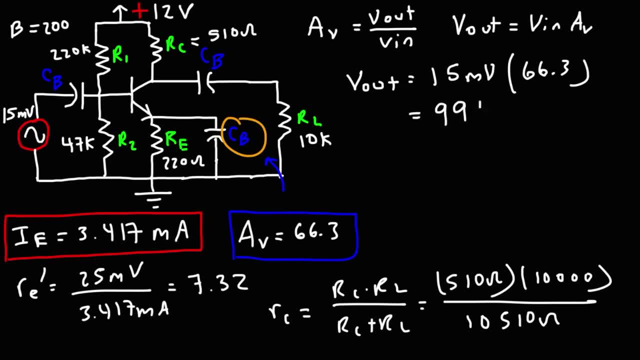 So the output voltage should be approximately 994.5 millivolts, or approximately 1 volt. So that's how you can calculate the output voltage, given the voltage gain and the input voltage. Now, one thing I do want to mention regarding the bypass capacitor. 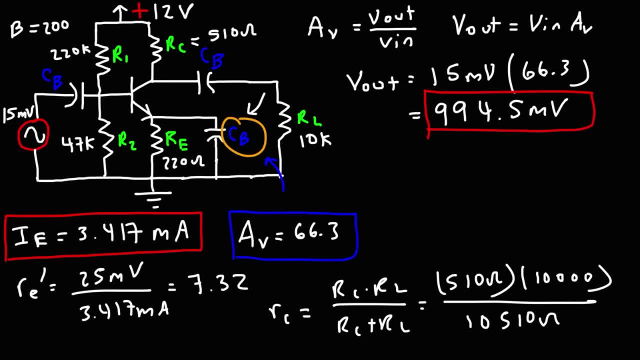 because I mentioned that adding the bypass capacitor decreases the overall AC meter resistance, which increases the voltage gain of the circuit, which is good. However, there is one drawback: Sometimes this can lead to distortion because the gain of the entire circuit, the voltage gain, is not stabilized. 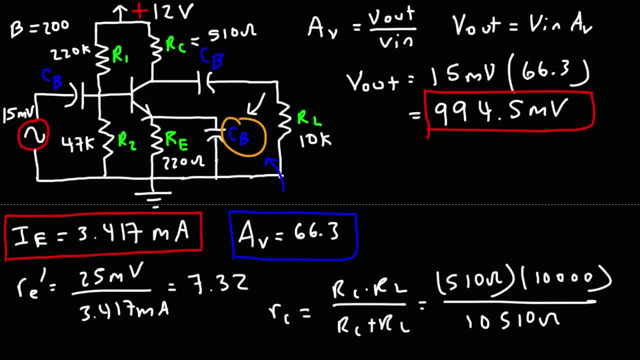 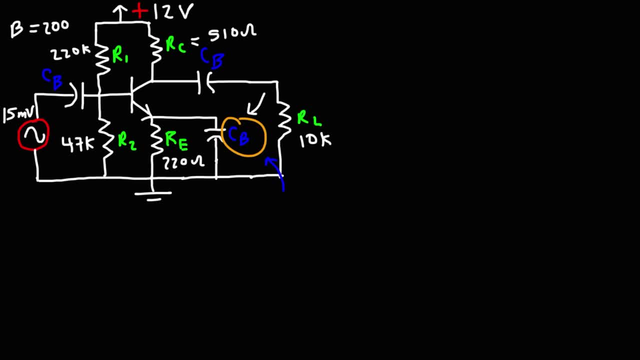 Let me explain why. So with the bypass capacitor present, the voltage gain is now RC divided by the AC meter resistance. Now let's say that RC is 1000, and the AC meter resistance is 4. This would be a voltage gain of 250. 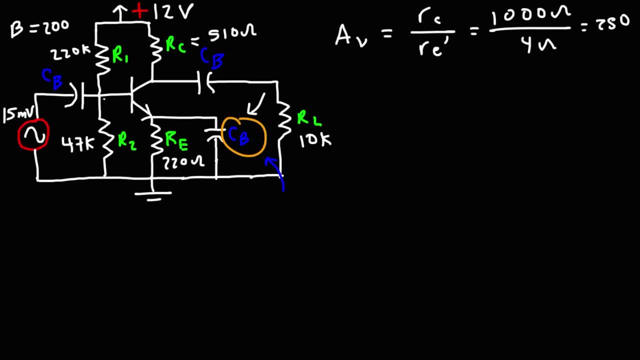 Now, as we have variations in the base current due to the AC signal, when the base current goes up, the emitter current will go up, because the base current is proportional to the collector current and the collector current is approximately equal to the emitter current. 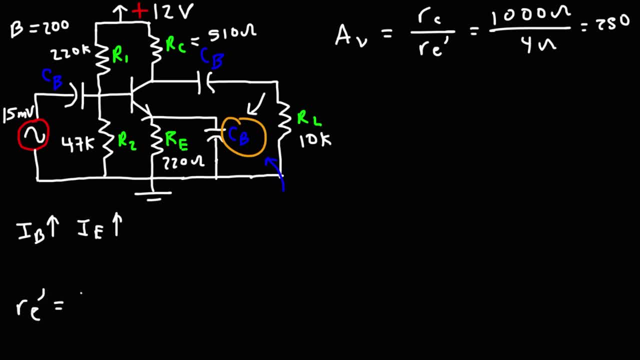 Now keep in mind, the AC meter resistance is 25 millivolts divided by IE. So it's inversely related to IE, which means that as IE goes up, the AC meter resistance goes up. I mean it goes down. Now that is inversely related to the voltage gain. 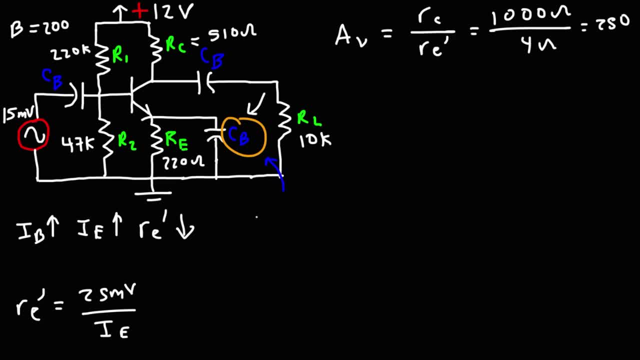 As the AC meter resistance goes down, the voltage gain goes up. So let's say, if IB doubles in value, That means IE is going to double in value approximately, And then the AC meter resistance is going to decrease by a factor of 2.. 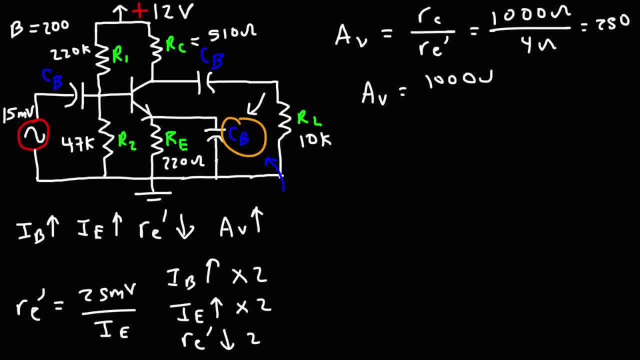 So if it decreases by a factor of 2, it's going to drop from 4 to 2, which means the voltage gain is 500.. Notice how much the voltage gain changed by from 250 to 500, which means it increased by 100%. 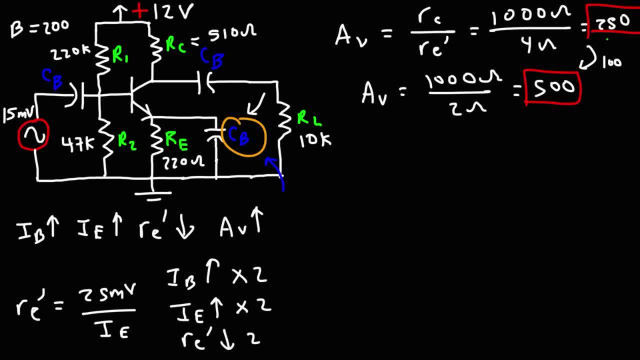 So that's huge. As you can see, the gain is not stabilized, But if we have a value for capital RE, notice, Notice how the gain is stabilized. So let's say, initially the AC emitter resistance is 4 and capital RE will say it's 50.. 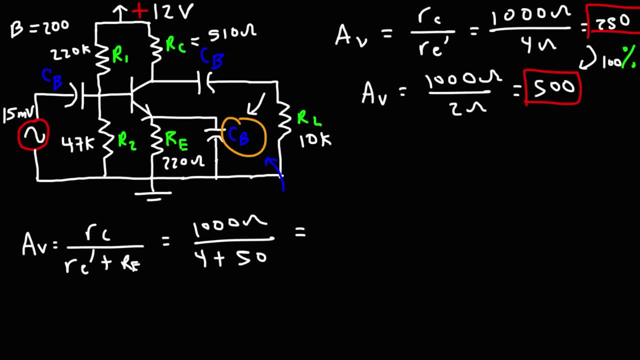 So this would be 1000 divided by 54.. So the gain will be 18.52.. Now let's say that the AC emitter resistance changes from 4 to 2.. Capital RE will be the same, And so now the voltage gain is 19.23. 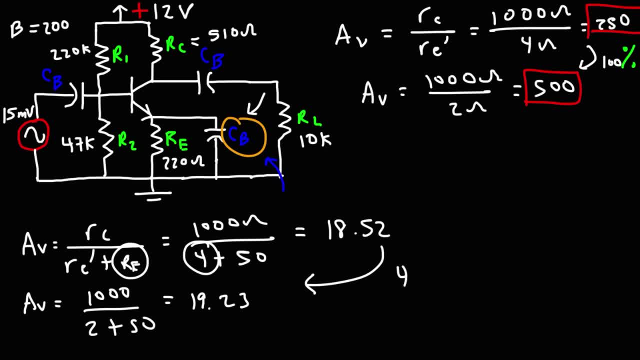 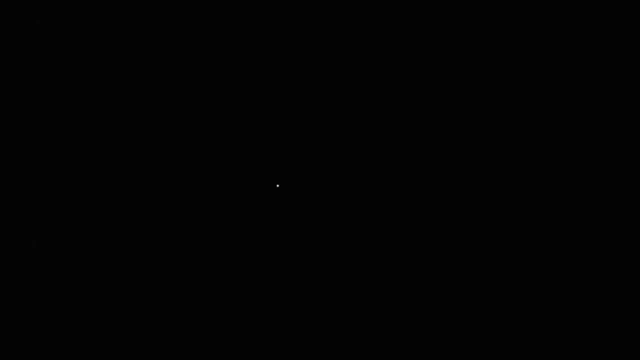 So that's an increase of approximately 4%, which is not that bad compared to an increase of 100%. So add in RE. So without the bypass capacitor, it stabilizes the gain. Now this is a special type of amplifier known as a swamped amplifier, which is a gain stabilized.